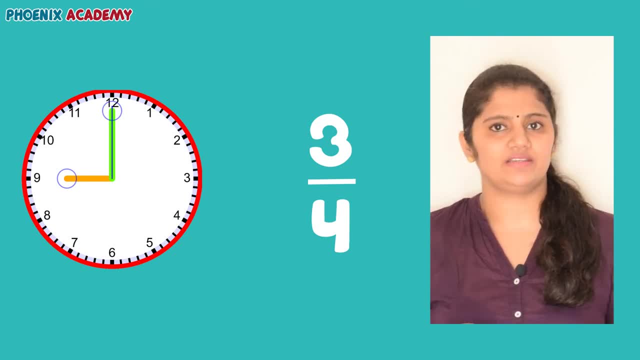 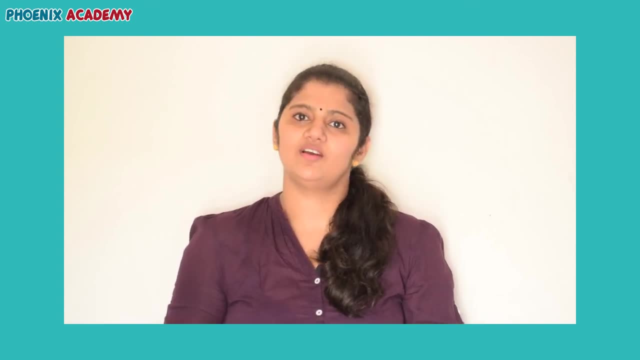 It is three-fourth or three-quarters. Today we have learnt fractions and how to identify what fractions of a whole. With a different topic we will see in the next session. I wish all of you a happy learning. 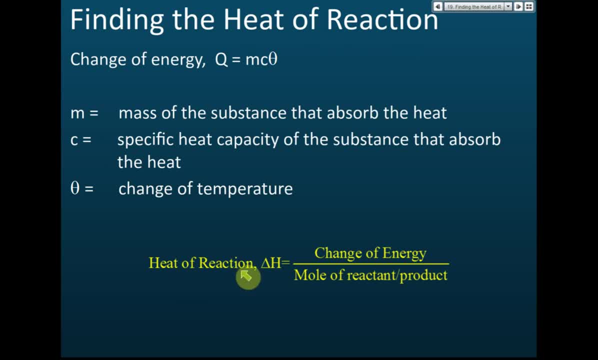 Finding the heat of reactions. Heat of reactions can be calculated by using this formula: The change of energy divided by the mole of reactants or product. Mole of reactants or product means the number of moles. Number of moles of the reactants or products. 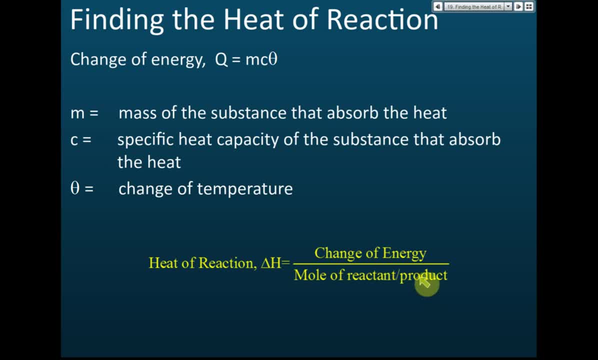 Now these reactants or products must be the substance, the reference substance in the reactions. For example, for heat of neutralizations we use water as a reference, Because heat of neutralization is the heat change when one mole of water produced. So then this mole of reactants or product must be the mole of water for heat of neutralizations. 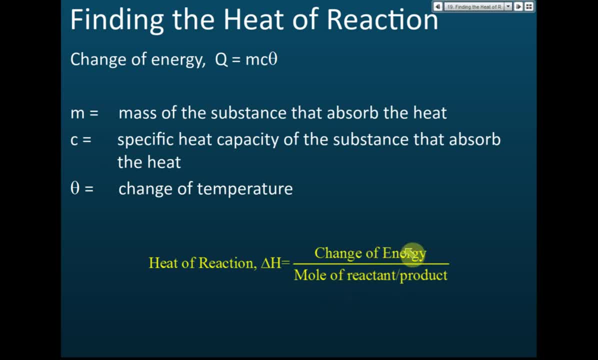 Then for the change of energy, we can calculate By using this formula- you should have learned this- in form 4.. Change of heat energy. Q equals to MC theta, where M is the mass of the substance. In our case, the substance is the solution. It will be the mass of the solution. 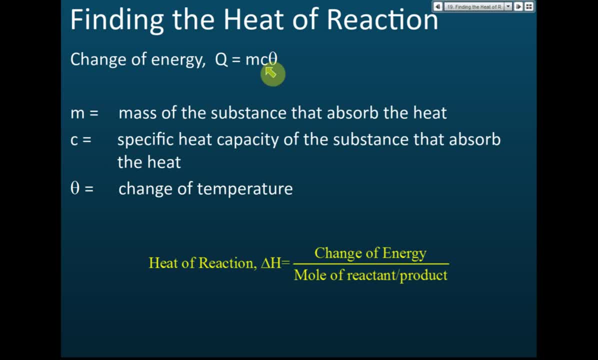 And C is the specific heat capacity. In chemistry usually the solution is water. So the specific heat capacity will be the specific heat capacity And zero is the specific heat capacity. cause: the mole of the substance cover the full system, wz will be the density of water and theta is the change of the temperature. 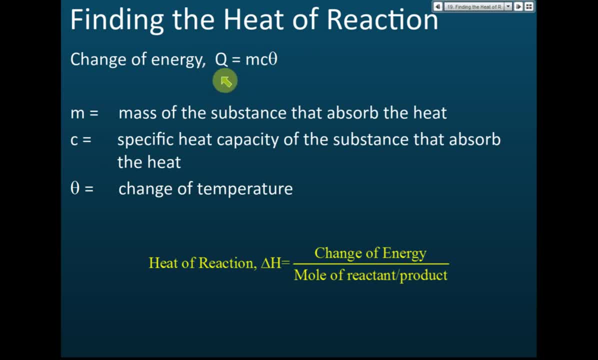 So we use this formula- Q equals to MC theta- to find the change of energy, and then change of energy divided by the number of moles of reactants or products, then we can get the heat of reactions. So that is how we find the heat of reactions. 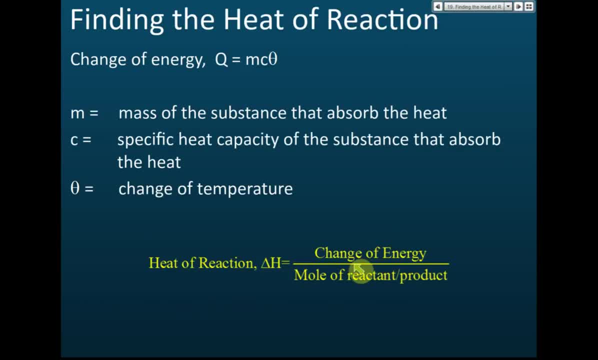 When we use this formula to find heat of reactions. there are a few things that you really need to know, And that's how we first find out about climate and six elements of temperature analysis. They are several points that we need to know, Okay.